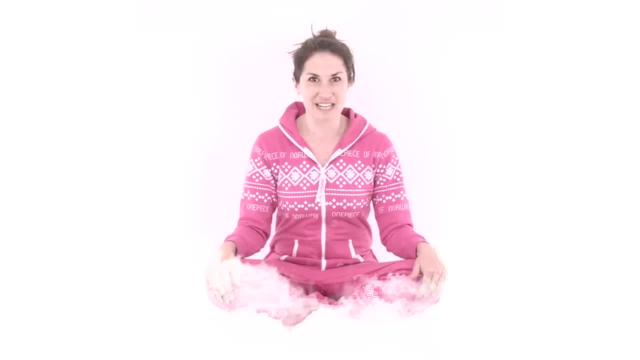 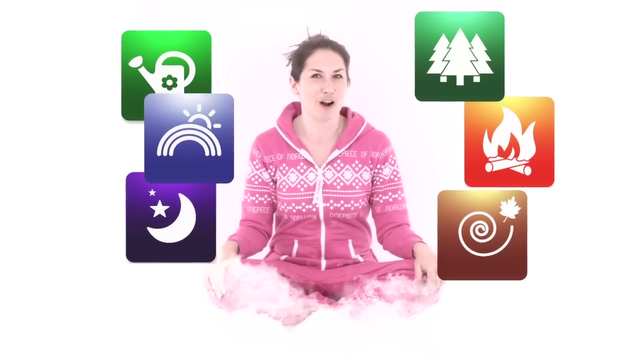 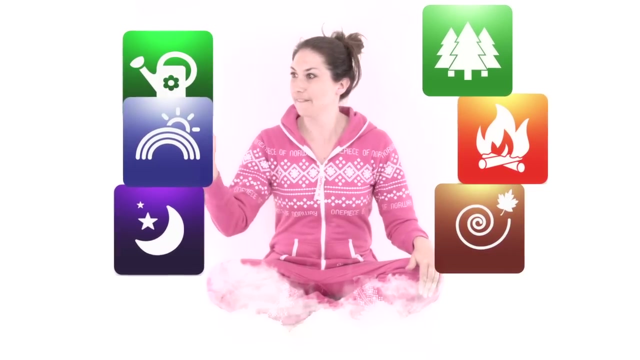 better. Now let's get the Zen Den ready so we can really enjoy it. We need music. Let's rub our ears and make the sounds appear. Well done everyone. that's done it You. now let's pick some that help us feel just right: The sound of a forest, A rainbow, The 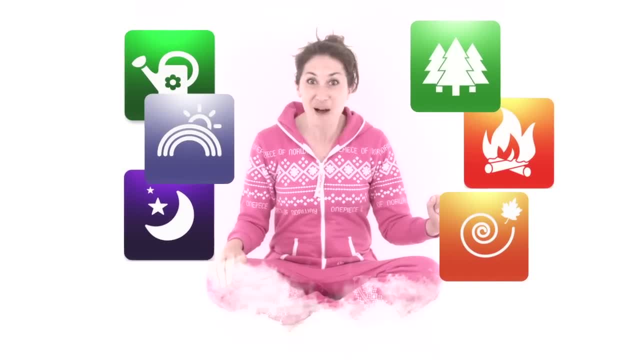 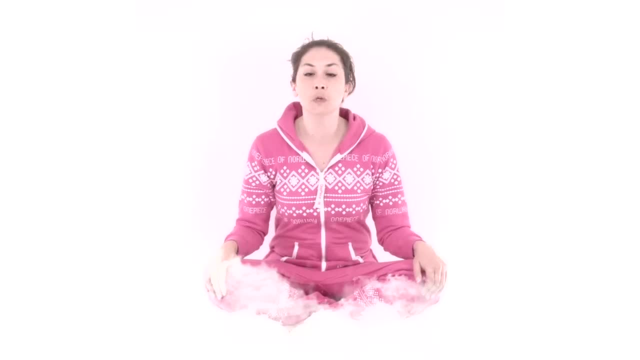 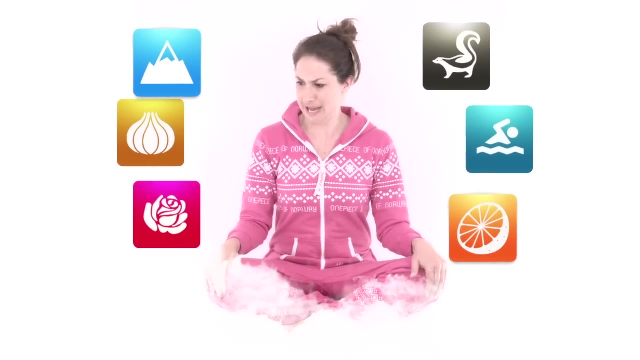 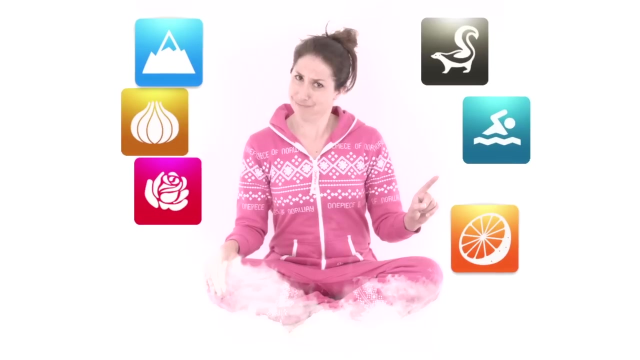 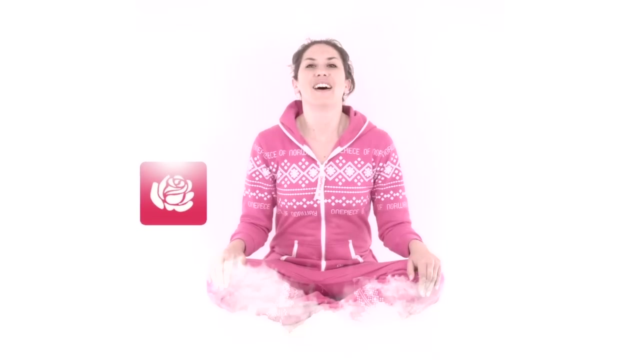 wind in the trees. Perfect, Now for the smell. Let's wiggle our noses. Oh yes, we did it. Brilliant work, everyone. What have we got here? Hmm, skunk smell Swimming pool. Oh yes, let's smell the rose. Ah yes, that's such a pretty smell. 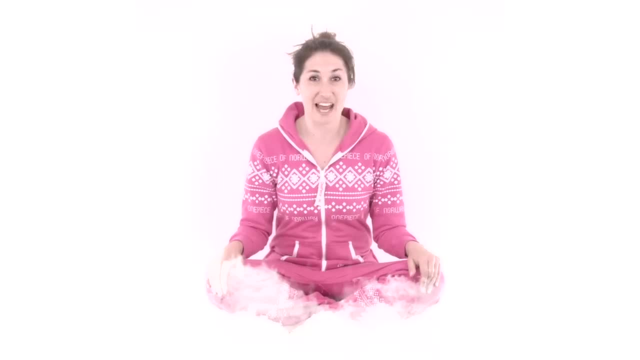 Today we're going to talk about something that happens to all of us. sometimes I call it getting wanty. Have you ever noticed, when you are in a shop or a store, how you look around and you see something that you want? Maybe you're in a toy shop and you spot something. 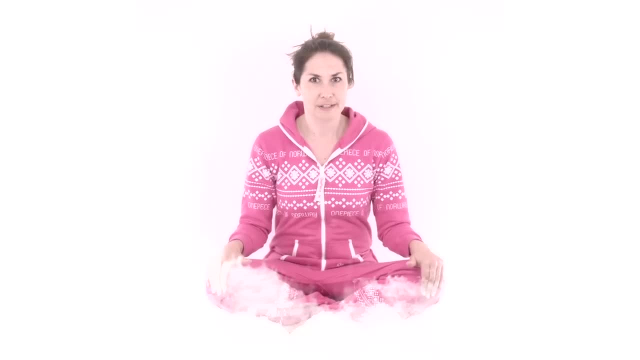 on a shelf and it's something you like the look of, and a little pop goes off somewhere inside you, making you really want that thing. You reach for it, take hold of it, look at it closely, maybe carry it around for a while, and then you want the item even more Now. 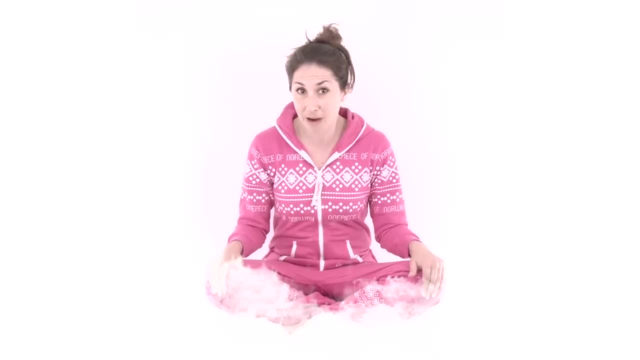 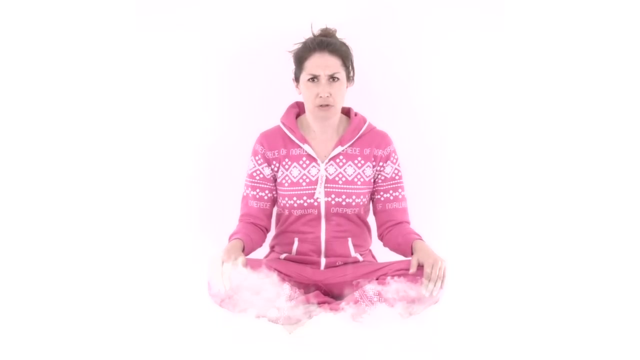 you look at it and decide that today the answer is no. Oh, when this happens, you feel something, don't you? Can you notice that feeling? You may feel disappointed, sad or even angry because of this. You want this thing so much, but you can't have it. 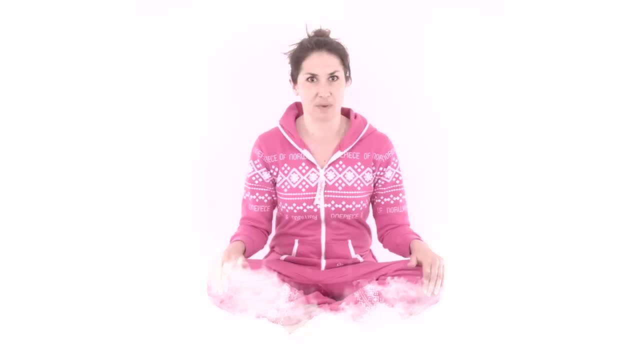 Maybe you want it even more now that you've been told you can't have it. You might think it's unfair that they are being mean for saying no to you. That is the wanty feeling getting bigger. At this point you have a choice. Hold out your hand and let's press the freeze.